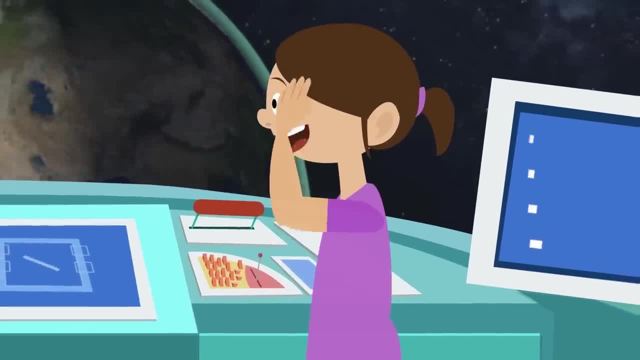 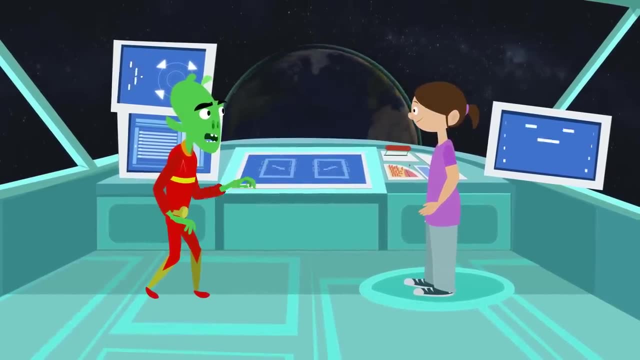 Can you explain them to me? Oh my, you did scare me. You're lucky, It was just a few days ago. we learned about eclipses in class. Awesome, Tell me everything about them. Okay, Very well, then Pay close attention. 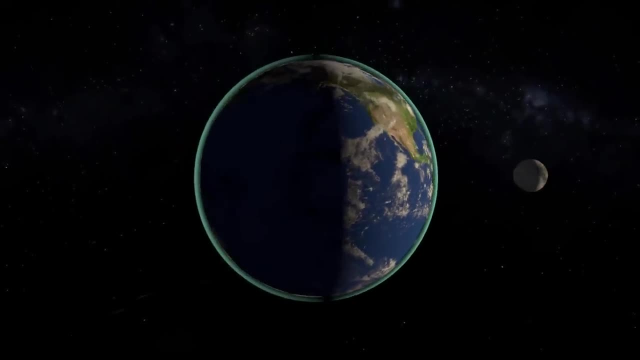 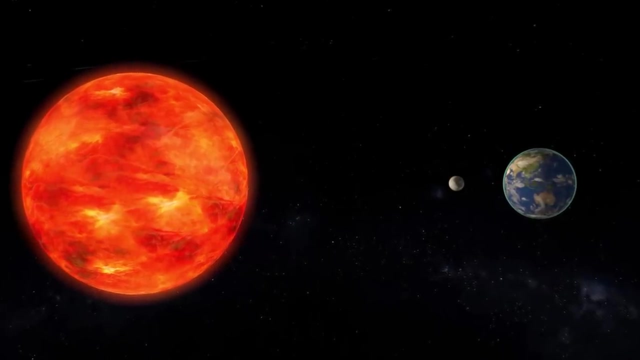 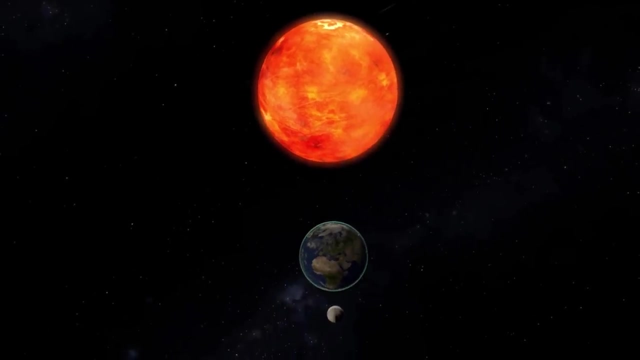 Sometimes the Sun, the Earth and the Moon align together, forming an eclipse On Earth. we can see two types of eclipses: Solar eclipse, like this one right here, and lunar eclipse, which would occur like this. I'll tell you about it step by step. 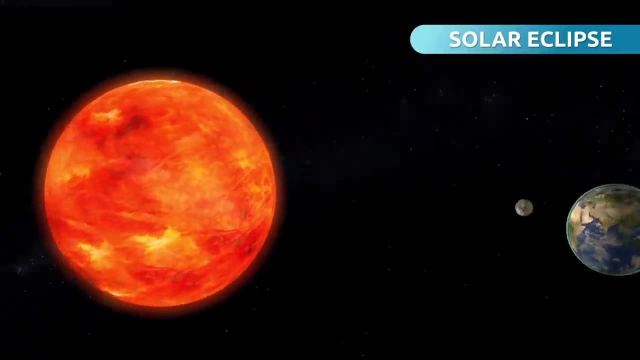 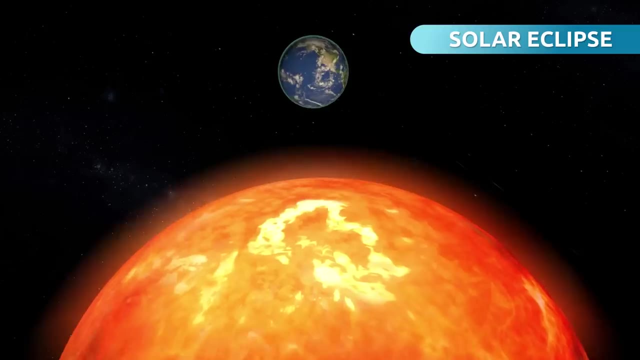 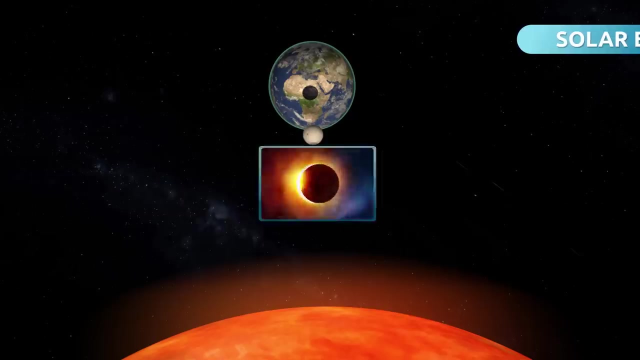 A solar eclipse is produced when the Moon comes between the Earth and the Sun, blocking part of the sunlight or even the entire Sun. This means that during daytime, the Moon positions itself in front of the Sun, covering it up. That's why, from Earth, we see something similar to a ring of light. 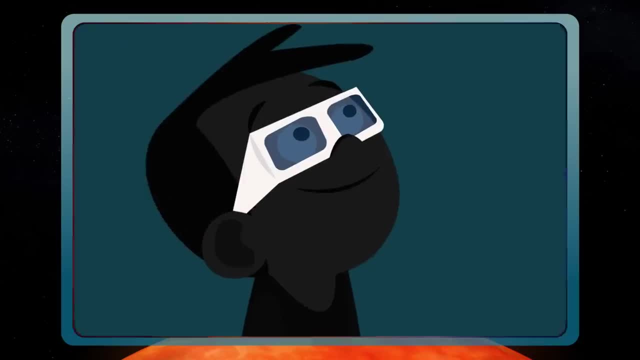 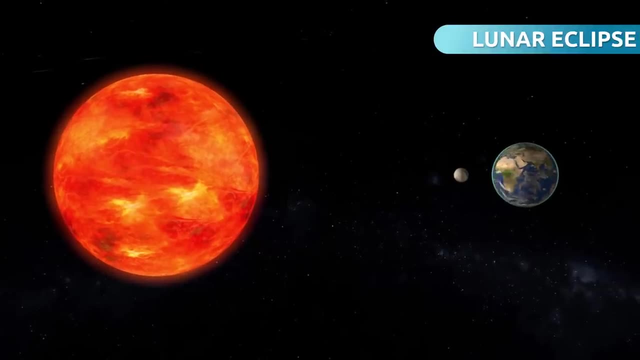 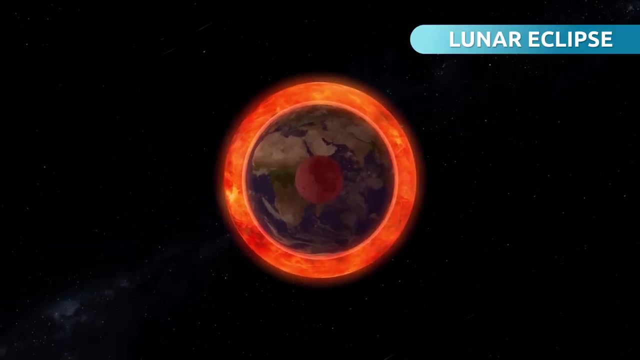 It's very important to know that to observe an eclipse, it's necessary to cover up your eyes using special eyewear. During a lunar eclipse, the Earth positions itself between the Sun and the Moon, blocking Sun rays from reaching the Earth. During the eclipse, a shadow is formed and the Moon becomes dark in our view, changing its color to red. 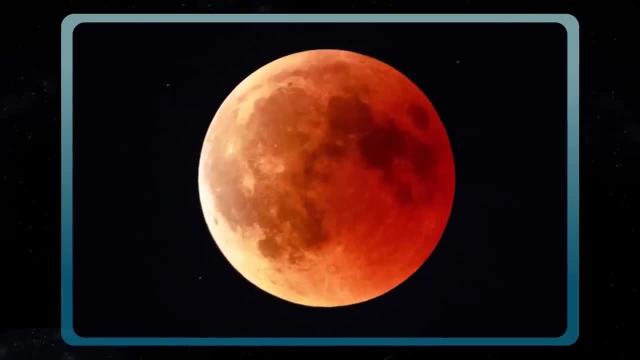 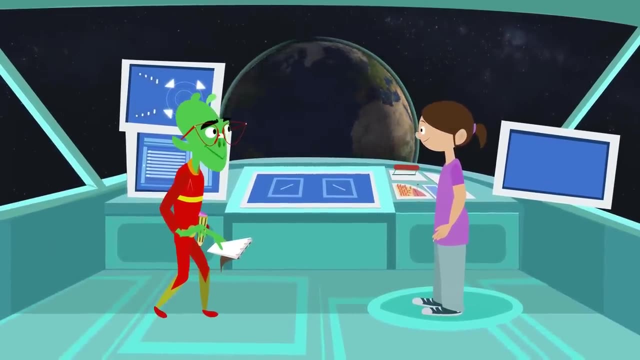 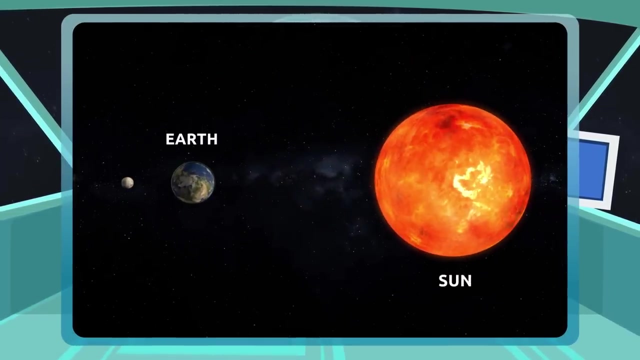 This phenomenon is known as blood Moon, And that's all about eclipses. It's very interesting, isn't it? It's incredible, Let's see. Read to me what you wrote to make sure you understood well. An eclipse happens when the Earth, Sun and Moon align together. 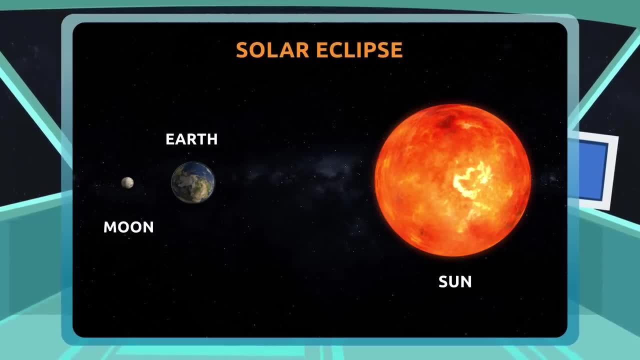 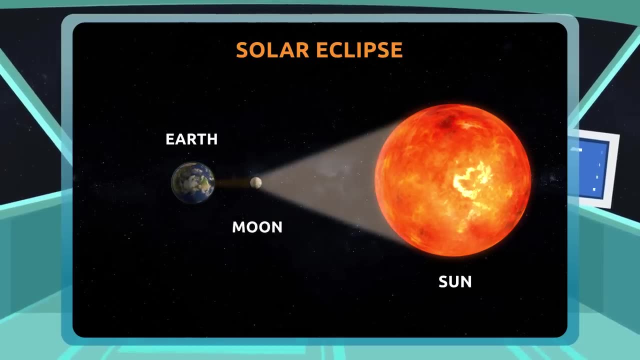 We can observe two types of eclipses. We can observe two different types of eclipses from the Earth. Solar eclipses occur when the Moon comes between the Sun and the Earth, forming a shadow that covers the Earth's surface. Lunar eclipses happen when the Earth comes between the Sun and the Moon. 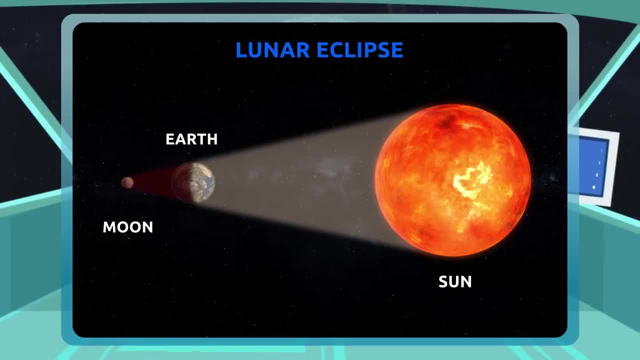 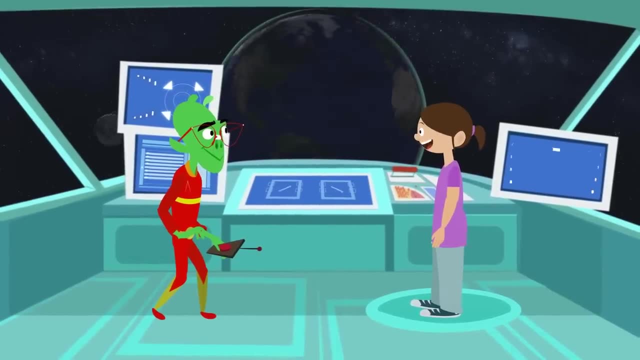 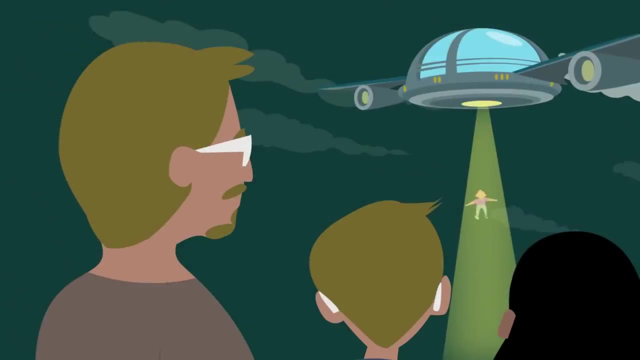 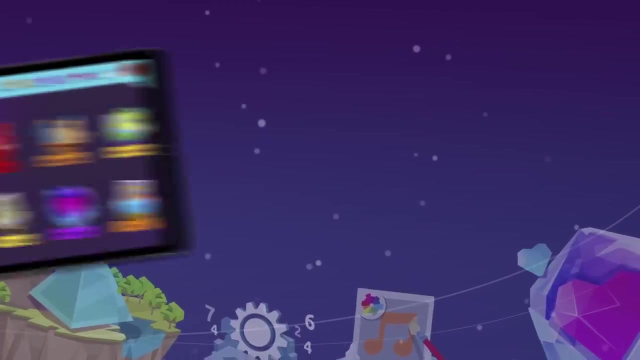 forming a shadow that covers the Lunar surface, changing the color of the Moon to copper red. That's amazing. You'll pass with flying colors. I need to get going. I have a lot of studying to do. You're very welcome. Do you want to keep on learning?